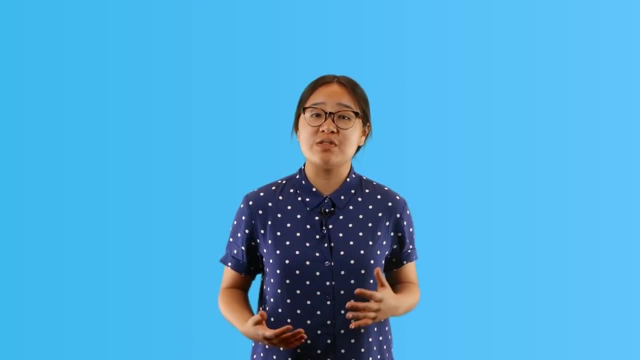 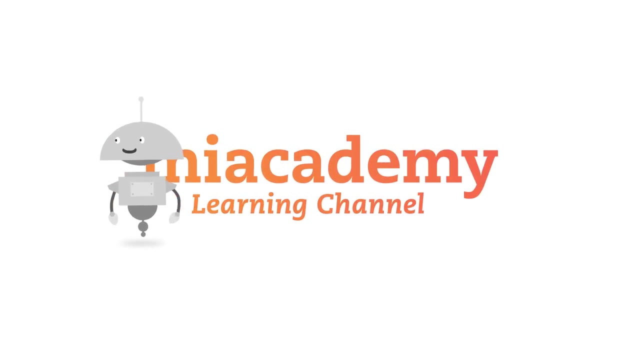 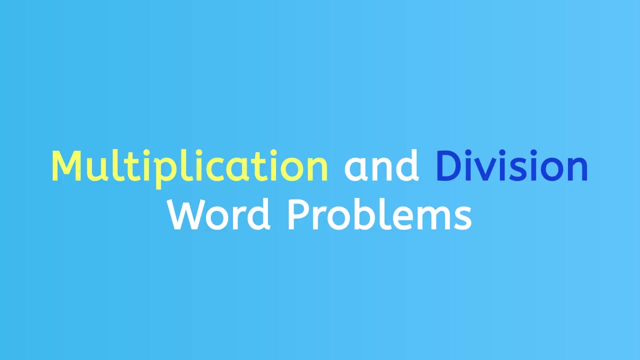 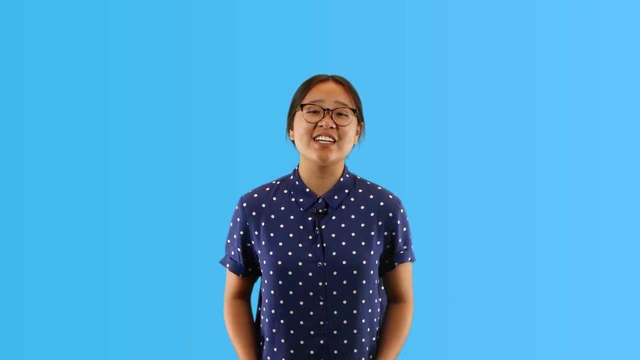 Hi, You've already learned how to do some word problems using addition and subtraction. Now it's time to learn how to use multiplication and division in word problems. Just like other word problems, these problems tell a story. The math problem is part of our story. 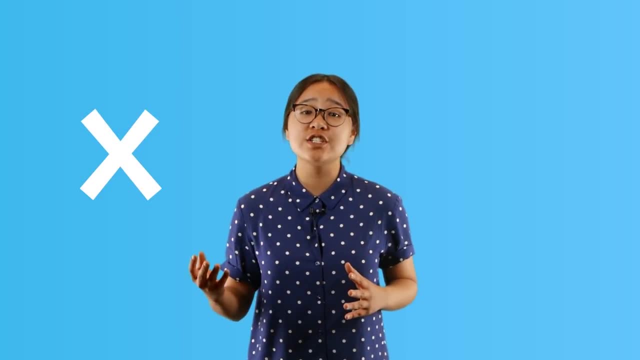 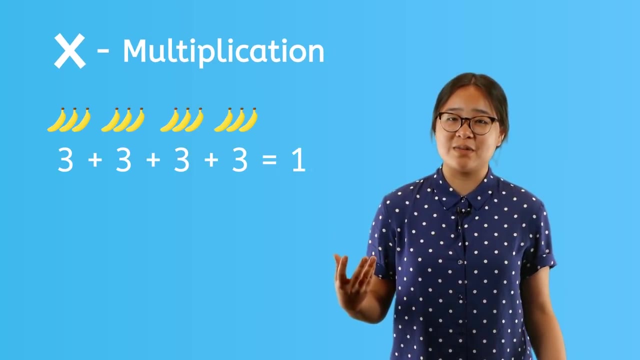 In this video all of the word problems will use multiplication or division. Remember, multiplication is a word that means multiplication. Multiplication is a word that means division. Multiplication is a word that means division. Multiplication is a way of adding together groups of numbers like a shortcut. 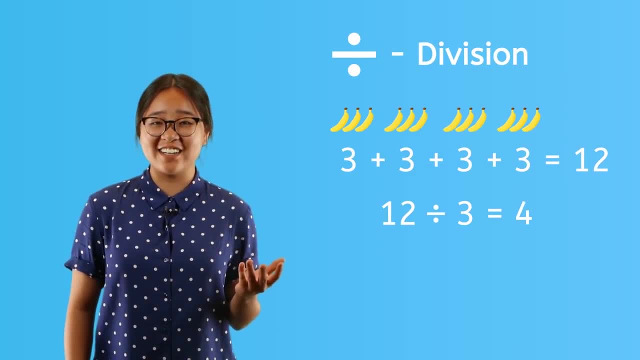 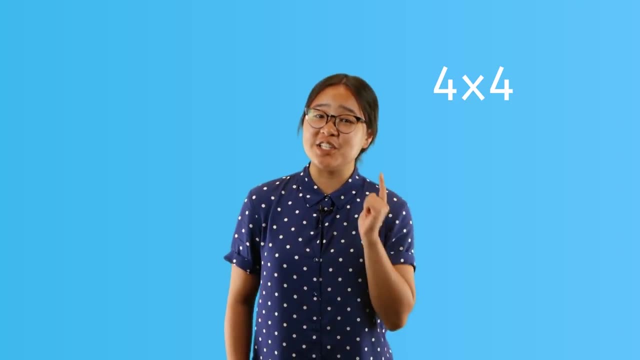 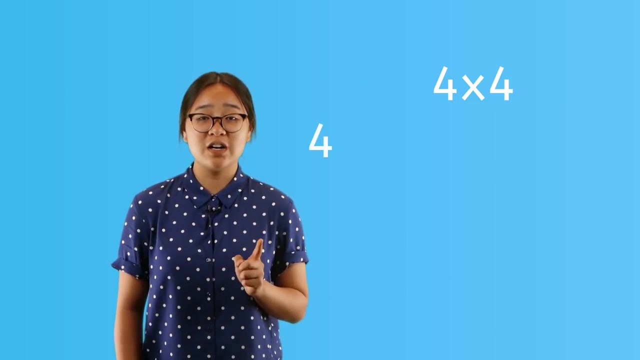 Division tells you how many groups of a number there are. Let's review what multiplication is. Start with four times four. Do you remember that four times four is four, fours or four plus four plus four plus four? Let's put that into a word: problem. 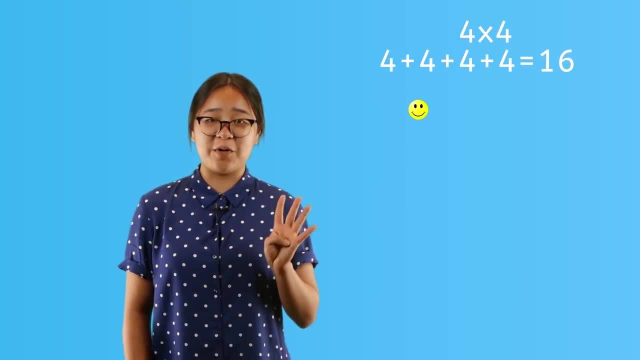 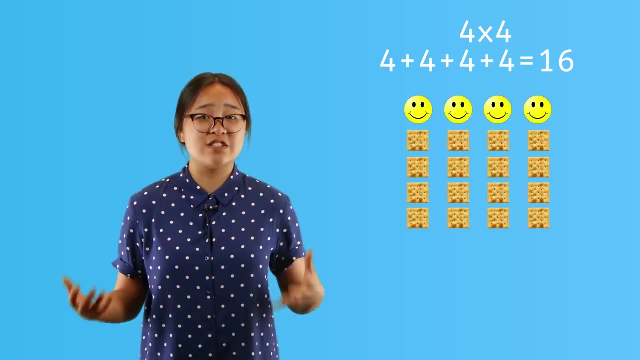 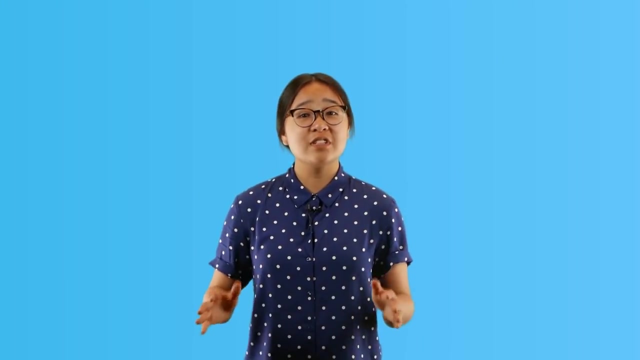 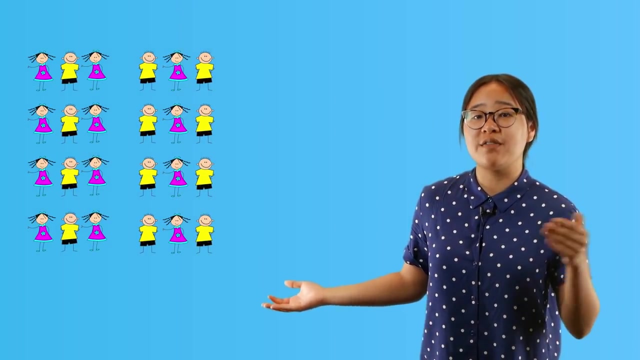 You are making a snack for four friends. You each need four crackers. How many crackers do you need? You'll need sixteen crackers for your snack. Now let's try another problem. During the field trip to the zoo, the class was divided into eight groups of three. 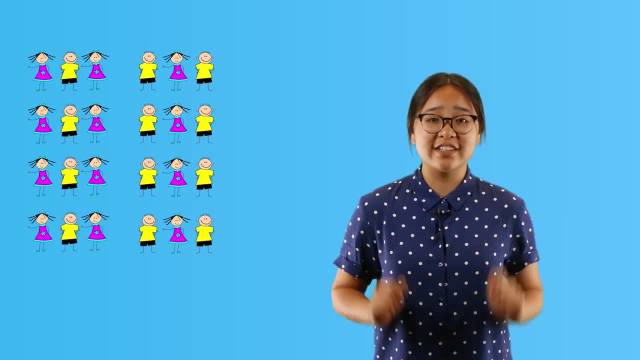 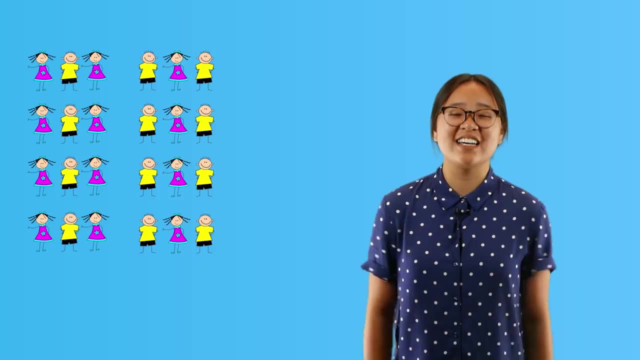 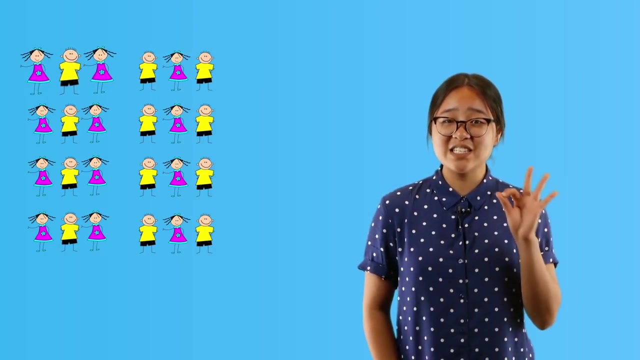 How many students are in the class. You are making a snack for four friends. You each need four crackers. How many crackers do you need? What do you need to do to figure it out? You need to multiply. We know that we have 8 groups and we have 3 students in each. 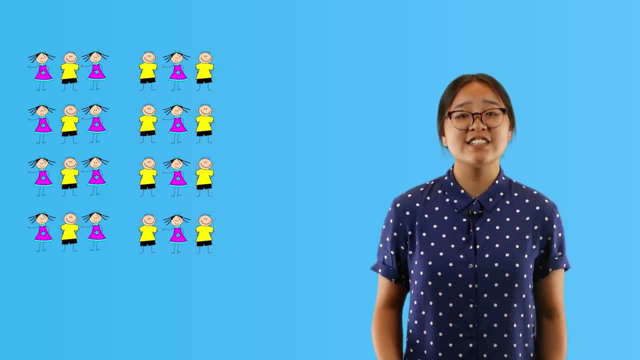 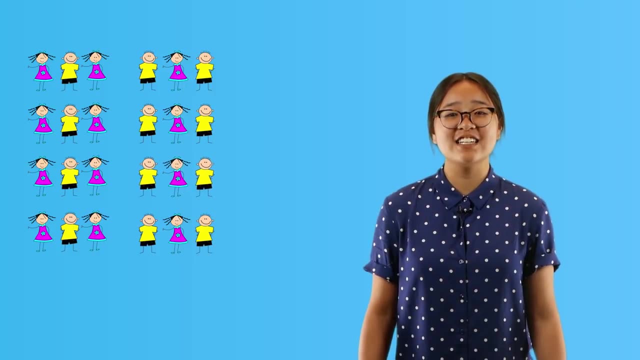 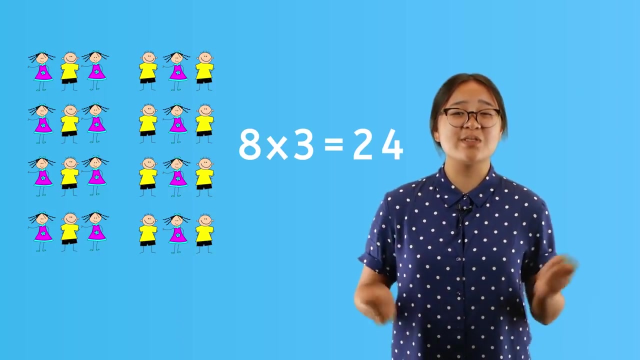 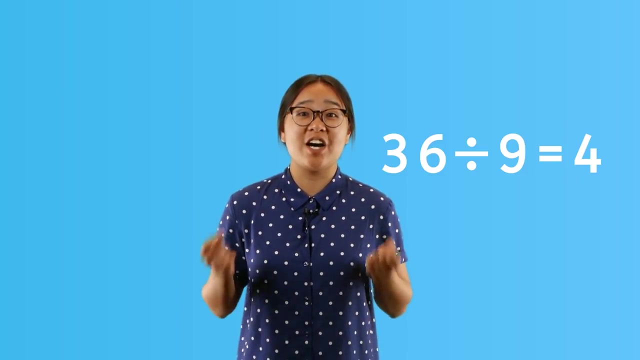 You can count them up: 3,, 6,, 9,, 12,, 15,, 18,, 21,, 24, but it's easier to just multiply. Do you remember how to divide? To divide, we are seeing how many groups we can make of a number.